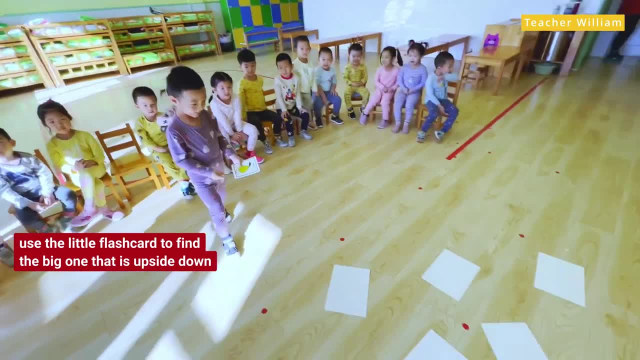 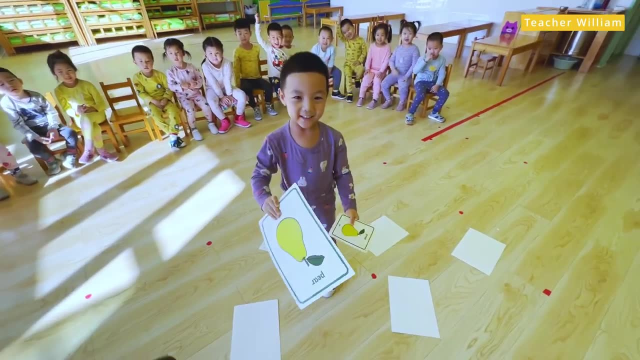 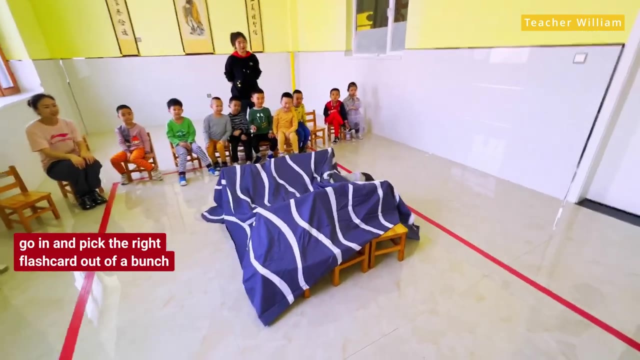 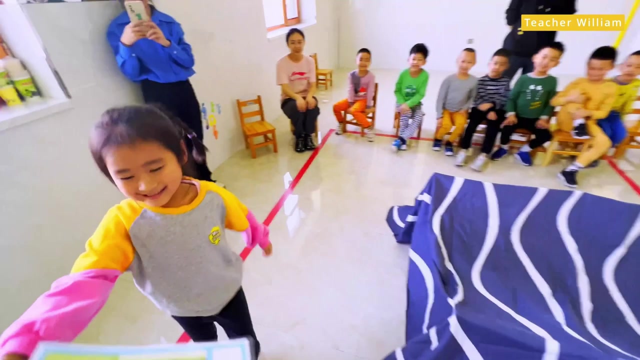 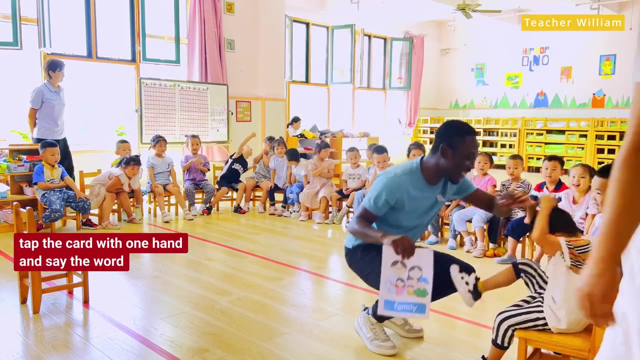 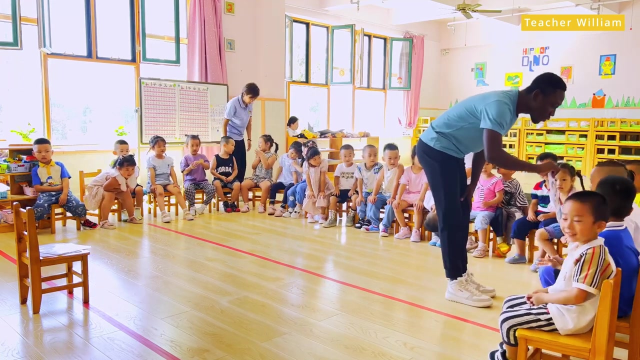 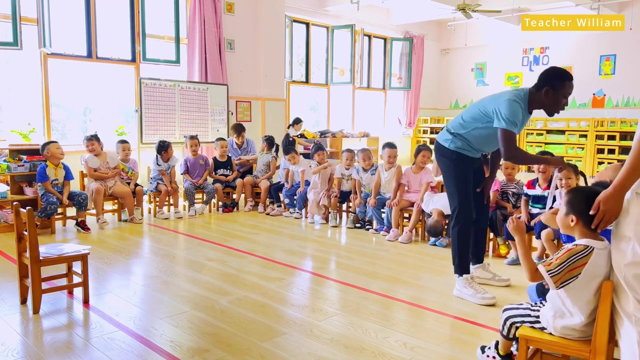 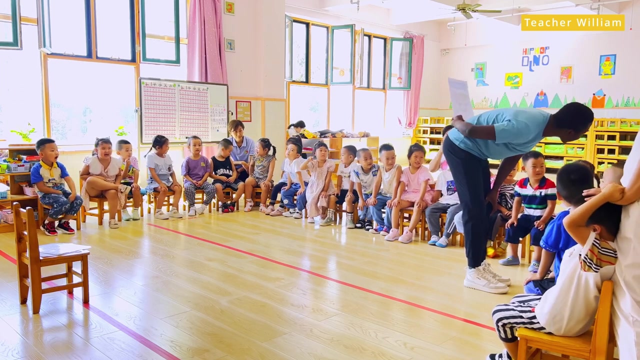 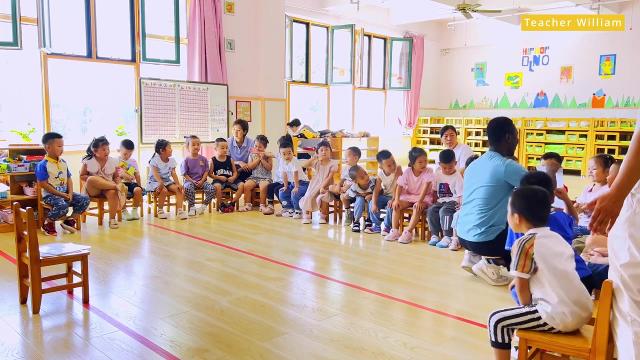 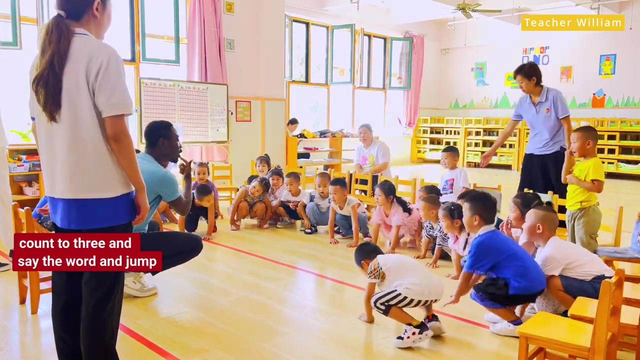 Very good, Look for pear Ready, Let's go Look for pear. Yay, Yay, Okay, very good, smart, okay. oh, ten, nine, eight, seven, six, very good, okay, let's say together: zoo, zoo, what's this? okay, one, two, three. 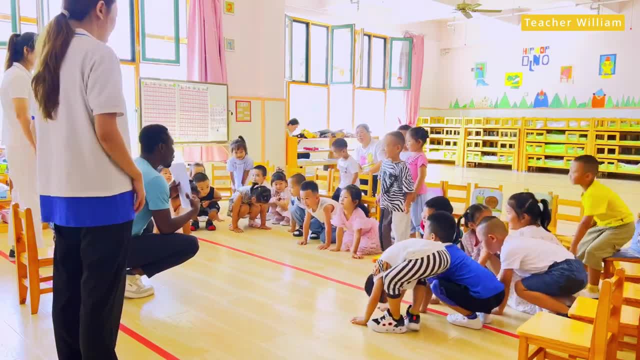 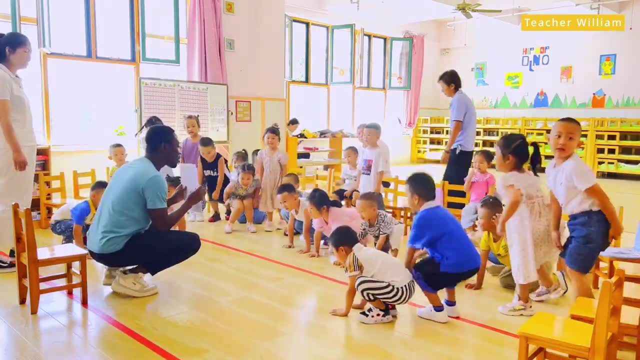 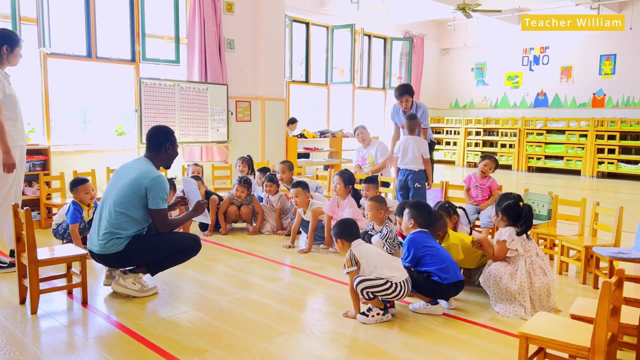 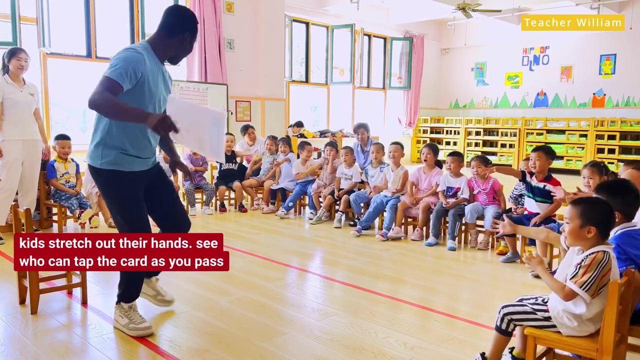 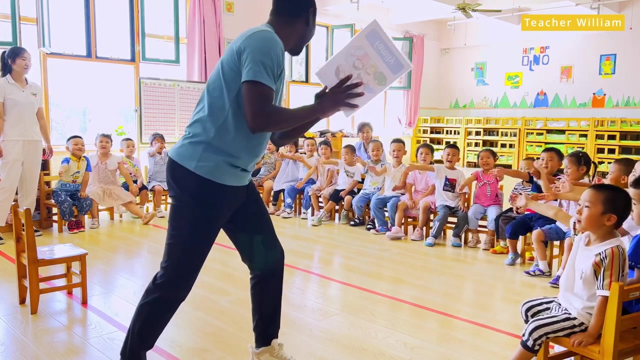 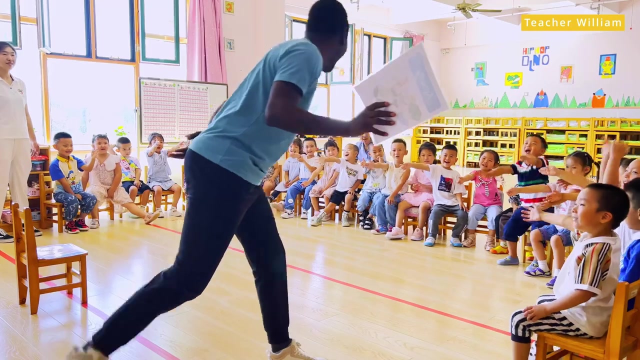 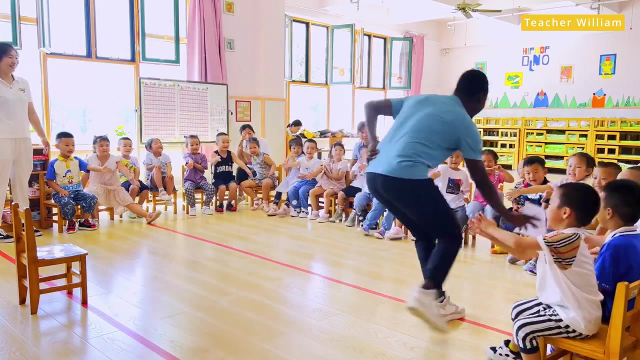 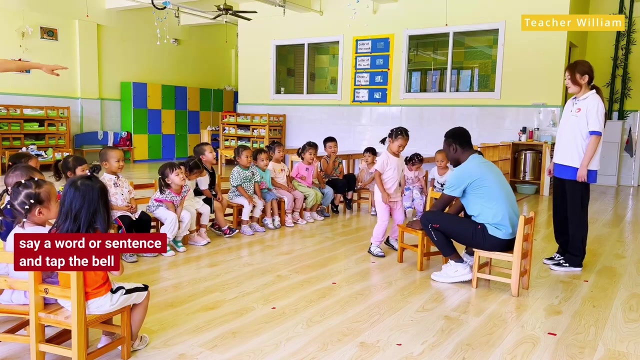 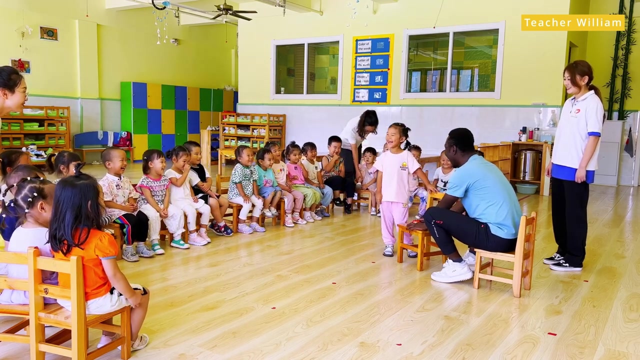 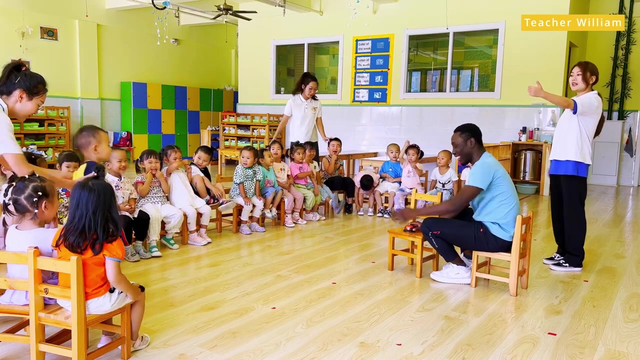 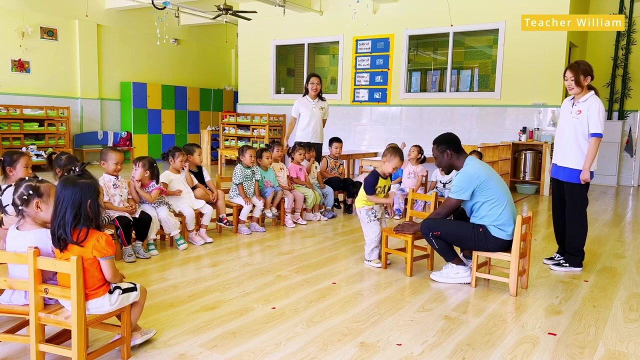 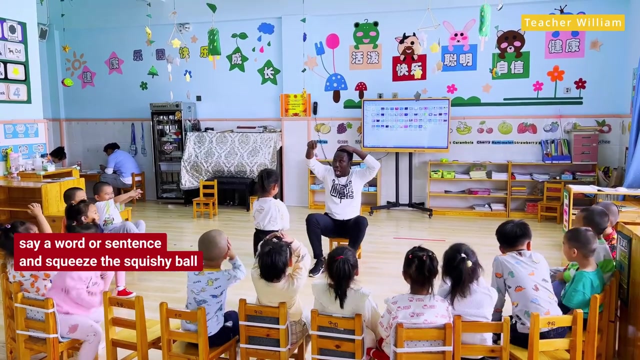 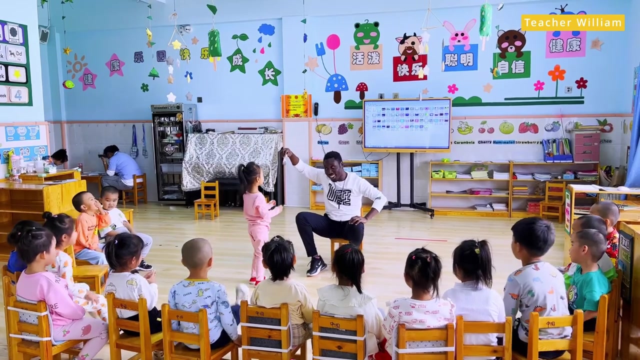 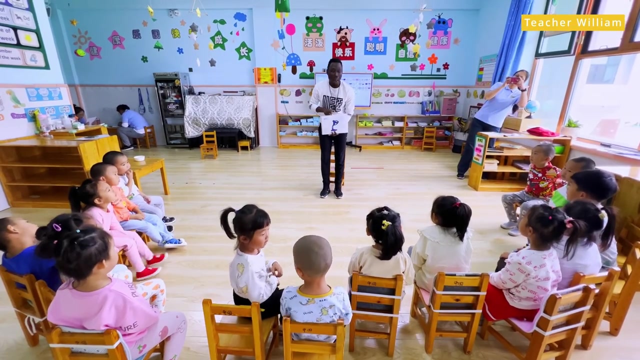 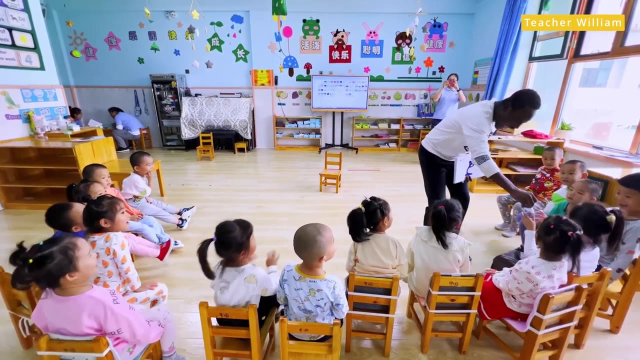 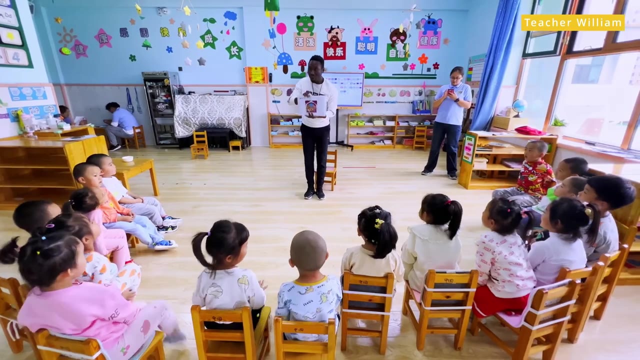 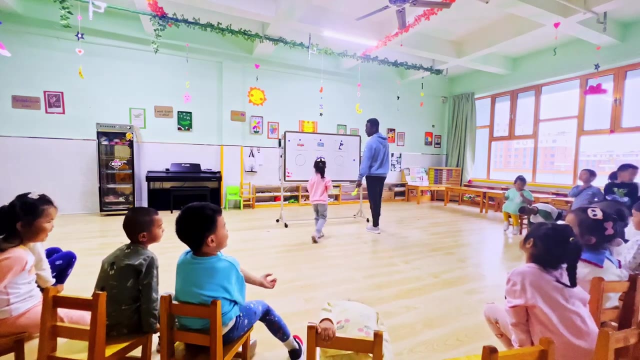 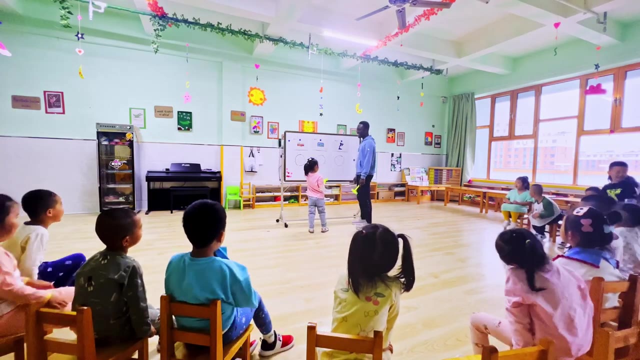 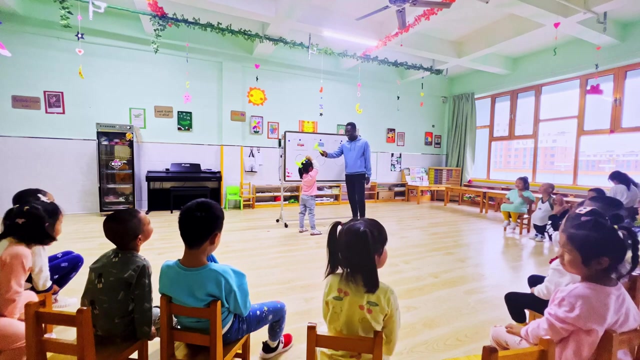 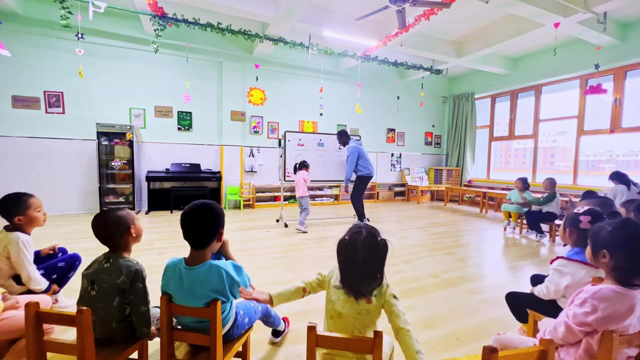 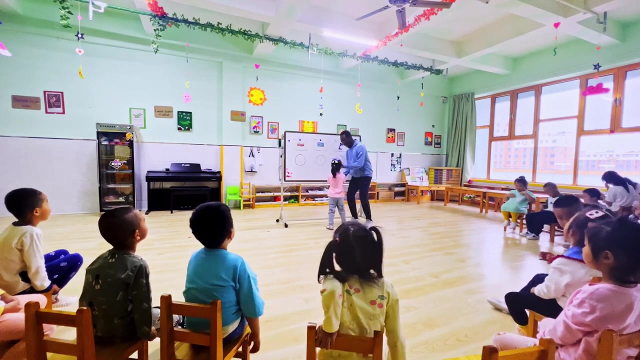 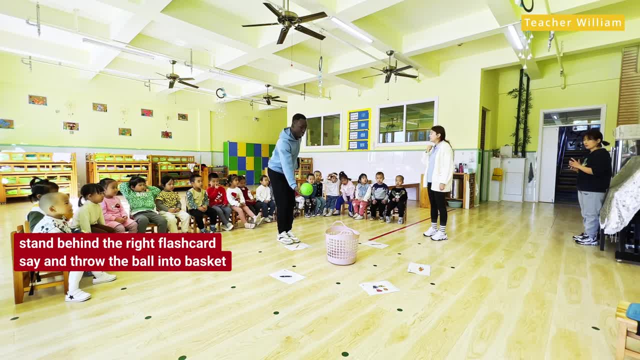 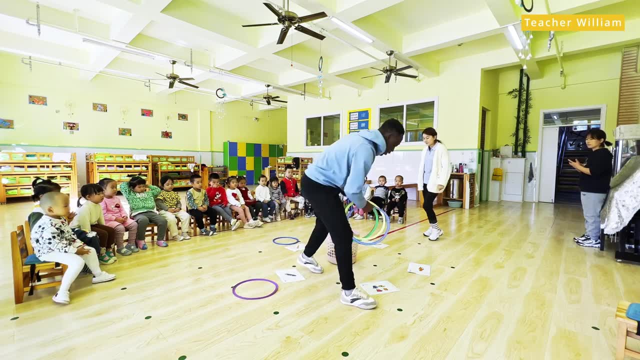 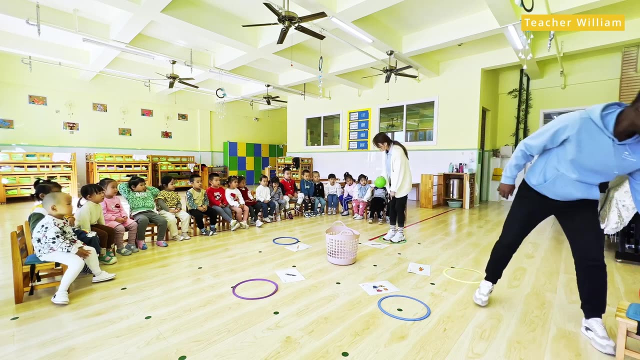 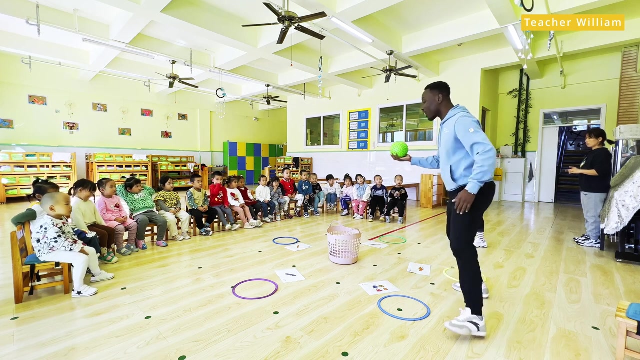 Okay. and then you throw the ball into the basket. Okay, Let me put it up here for you, Okay, Okay. and then you throw it into the basket. Okay, When Tita Williams says crayon, you look for crayon. 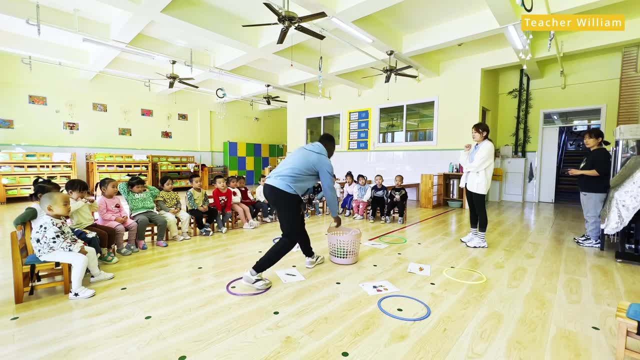 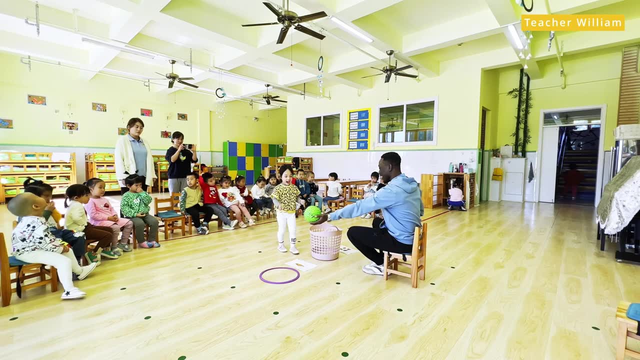 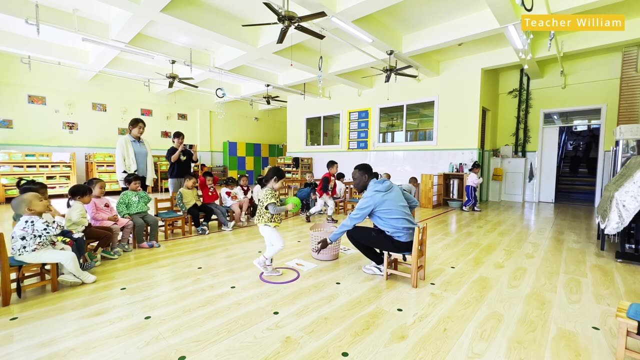 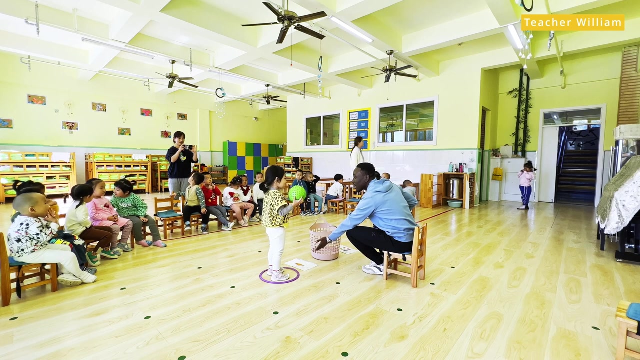 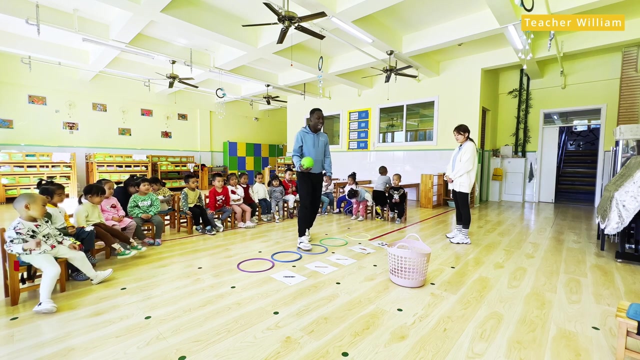 And then you throw the ball into the basket, Okay, And then I say book, And then you look for book, And then you throw the ball. Okay, And then you look for pen, And then you throw the ball. Okay, Okay. 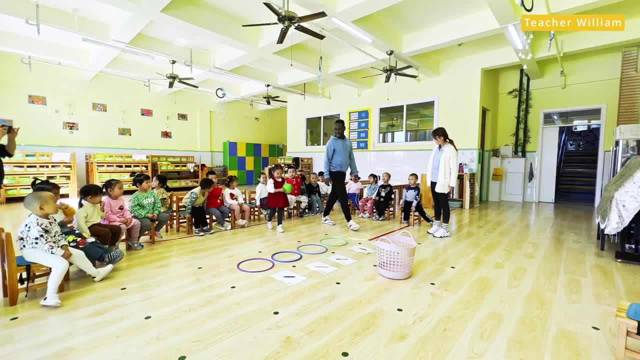 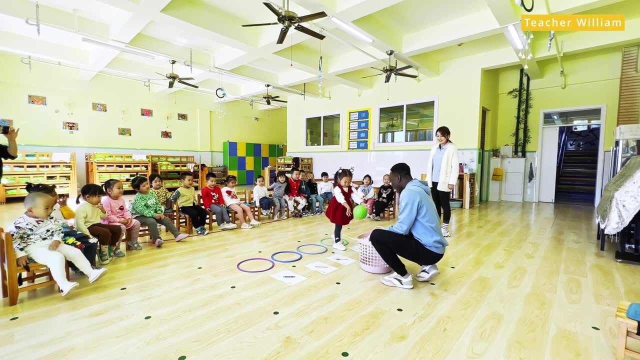 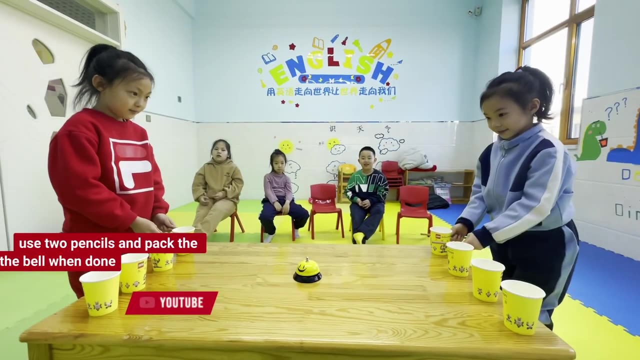 Okay, Very good, Book Book Very good. Okay, Go Press And say: book Book Very good, Good, Okay, High five, High five, High five, Ready, Ready, Go, One Go, go go. 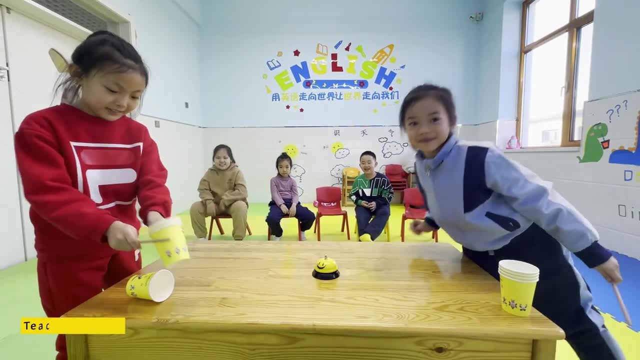 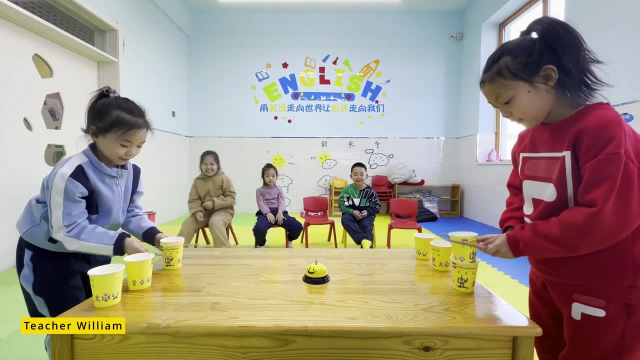 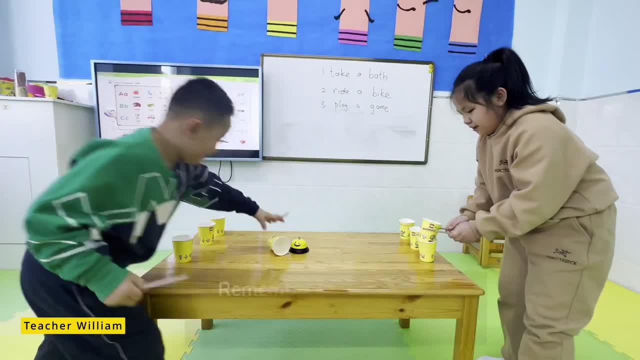 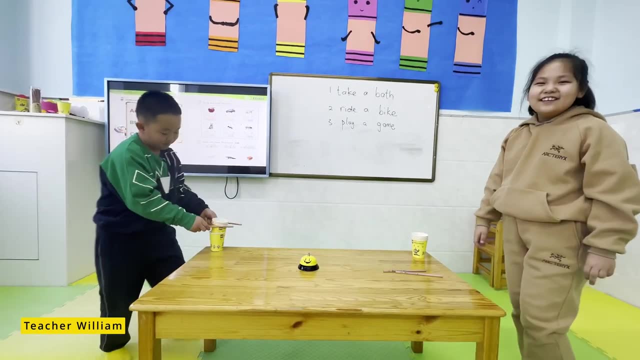 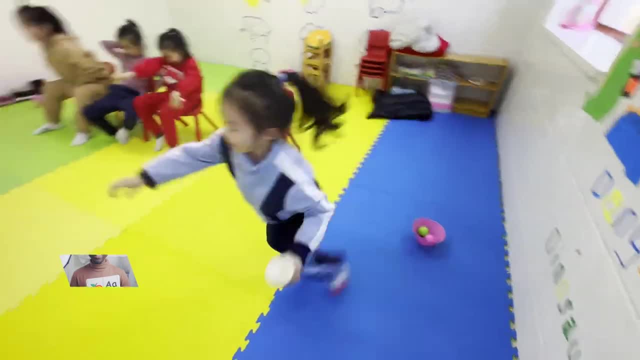 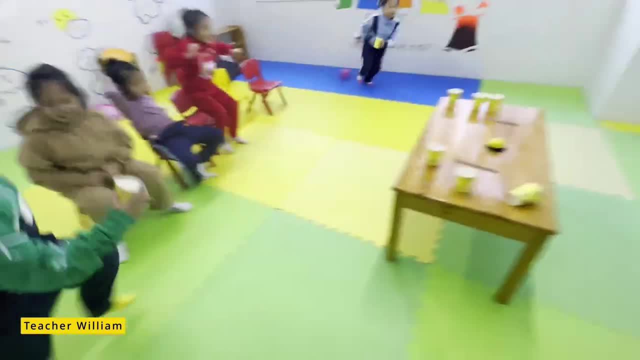 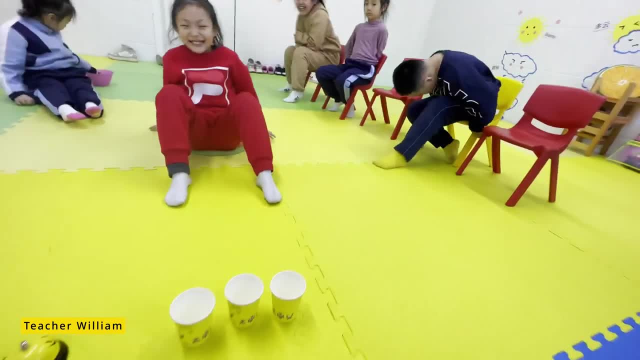 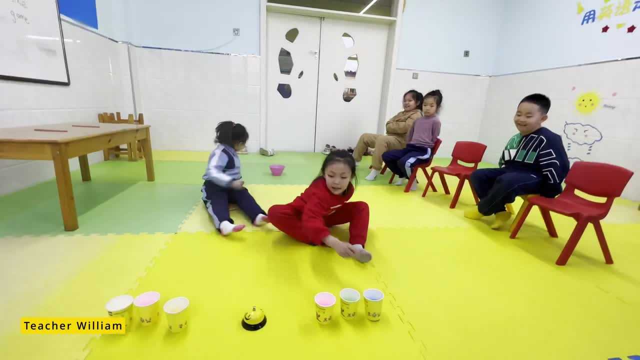 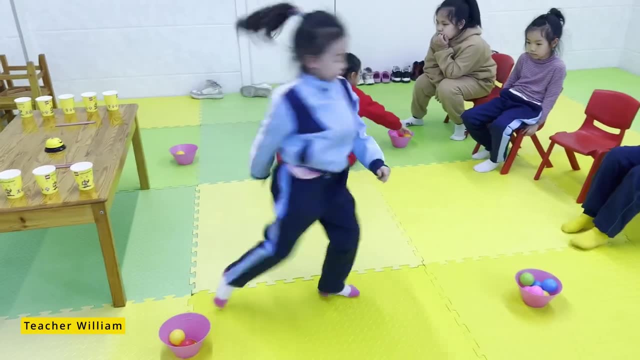